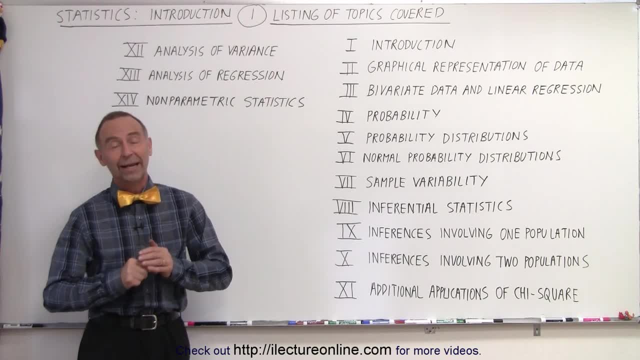 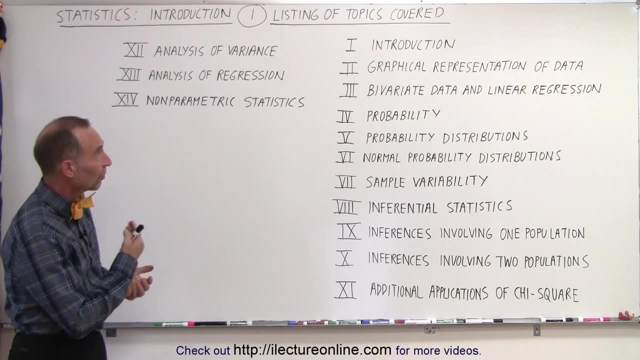 hmm, maybe doing some videos on statistics might not be a bad idea. So here we are. These are the topics that I'm planning on covering regarding statistics, And so the topics are: a basic introduction to statistics, the graphical representation of data, the bivariate data. 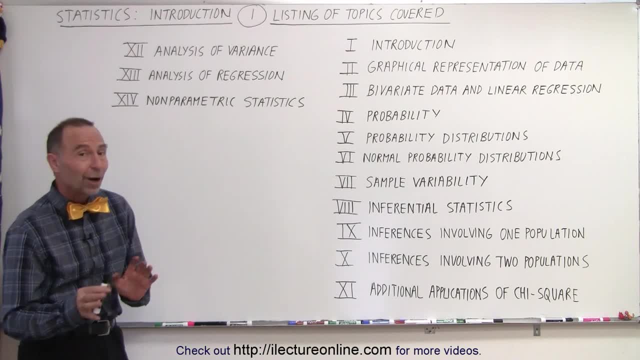 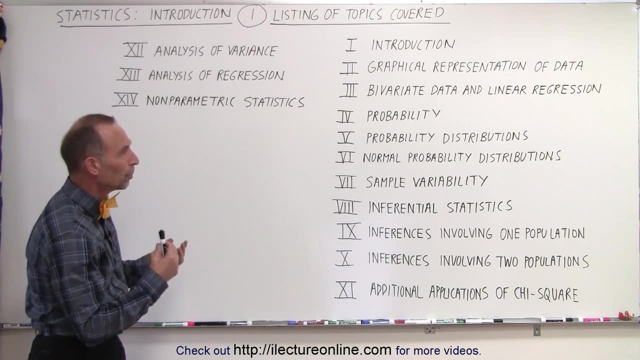 and linear regression probability. and yes, we are going to do some probability within statistics because there's a close correlation there- probability distributions, normal probability distributions. Then we do sample variability inferential statistics: inferences involving one population and inferences involving two populations. additional applications of xi squared. 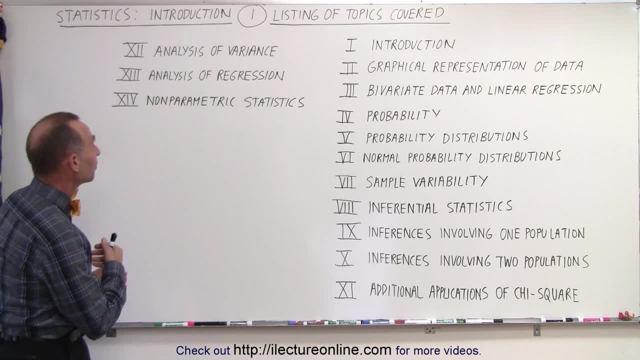 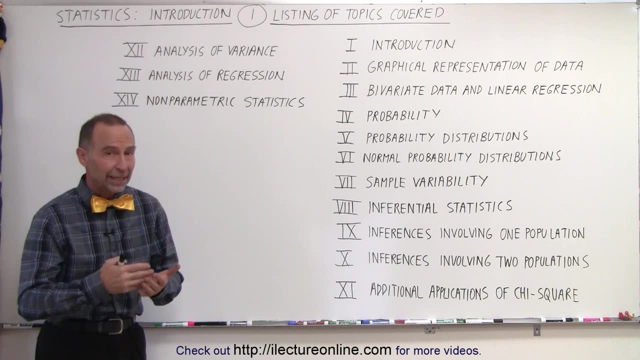 analysis of variance, analysis of regression and non-parametric statistics, And those are your basic topics about statistics. Statistics, of course, can get very complicated at higher levels. Maybe in the future we might cover those as well. But let's start with the more basic topics that 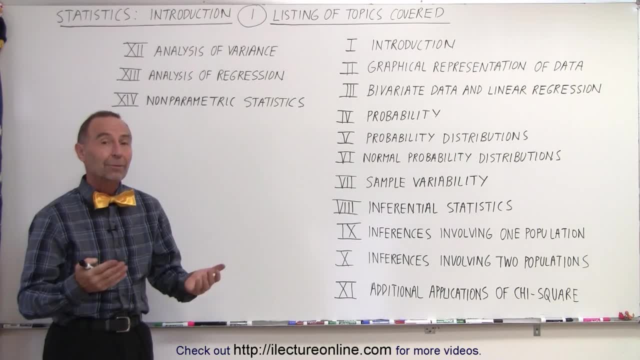 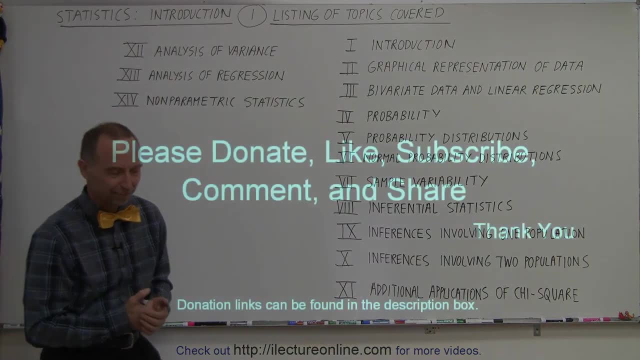 most of us need to know if we're doing any sort of work in mathematics or with statistics, And that is it. That's what we're going to cover in statistics. Thank you. 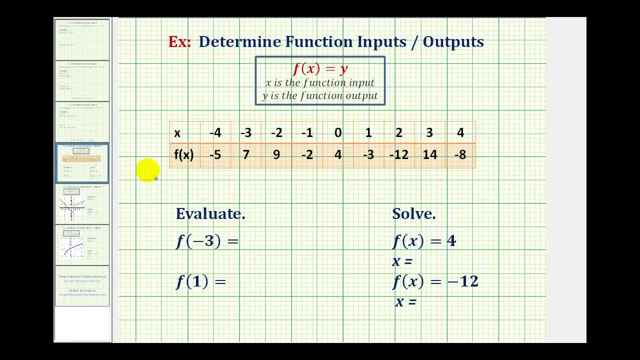 In this example we have a table that represents our function f of x, and then we're asked to evaluate function values and also to solve for x given a function value. When working with function notation, it's important to remember that f of x is equal to y, where x would be the input for the function and y would be the output of the function. 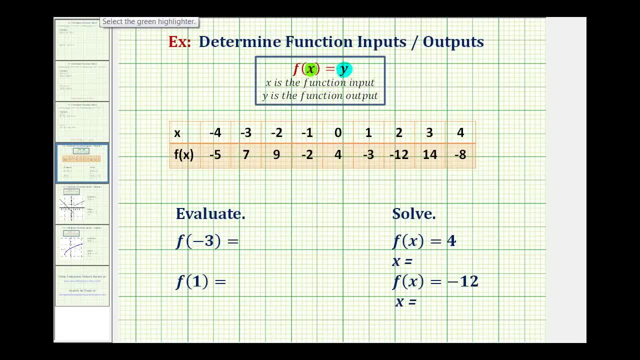 So to evaluate f of negative 3, we need to recognize that negative 3 is the x value and this function value is going to be the corresponding y value. So we're going to go to our table, which represents our function, and look for an x value of negative 3.. 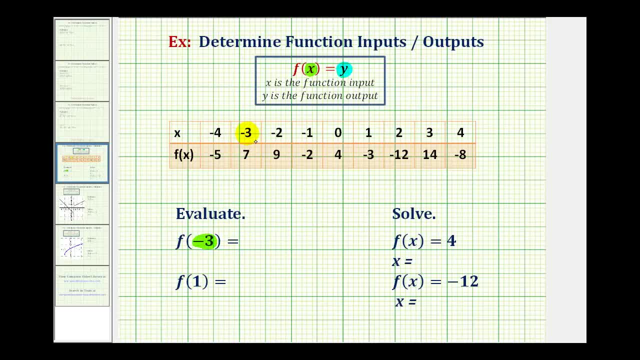 Notice, here it is, and the corresponding y value or function value is the function value we're looking for. So f of negative 3 is equal to positive 7.. Notice, if we wanted to graph this, we would have to do this.